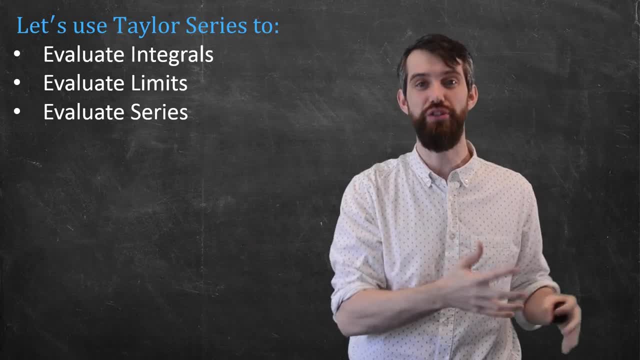 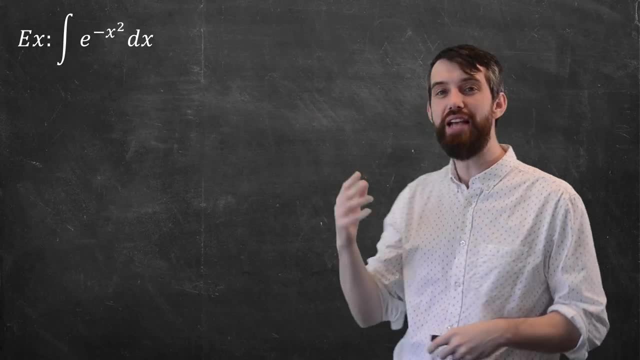 But now that we know Taylor Series, we can go back and do them. The first of these I'm going to focus on is an integration problem In particular. consider the integral of e to the minus x squared dx, and it's actually a very important integral. 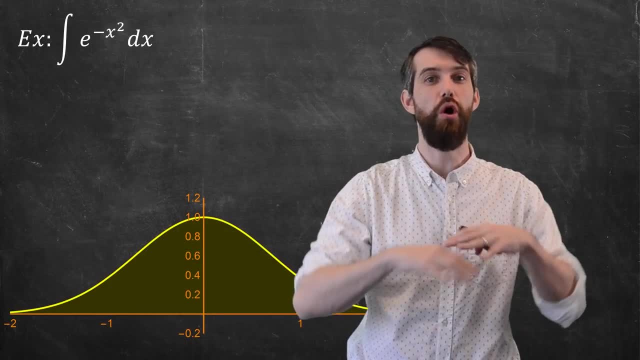 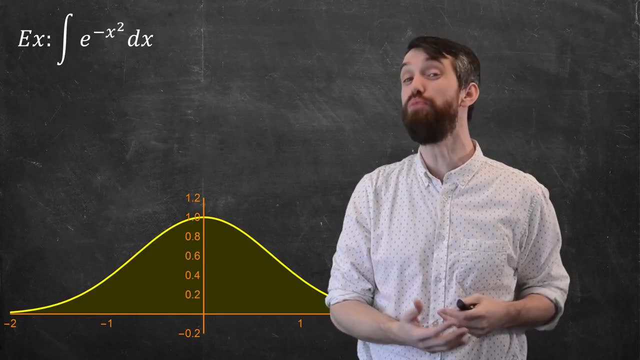 This kind of distribution in probability and statistics is called a normal distribution. It comes up all the time. So the issue of doing integrals of this form are actually pretty important, but we don't know how to do that by the methods of Calculus 1 or Calculus 2.. 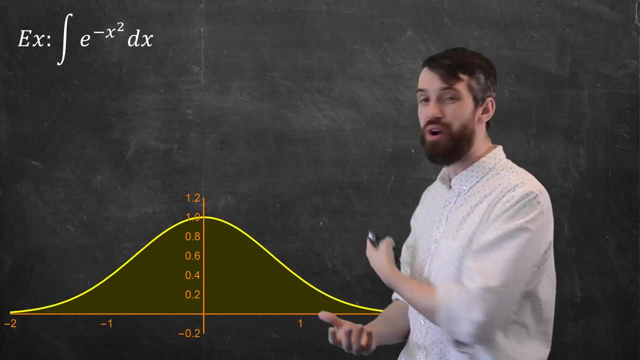 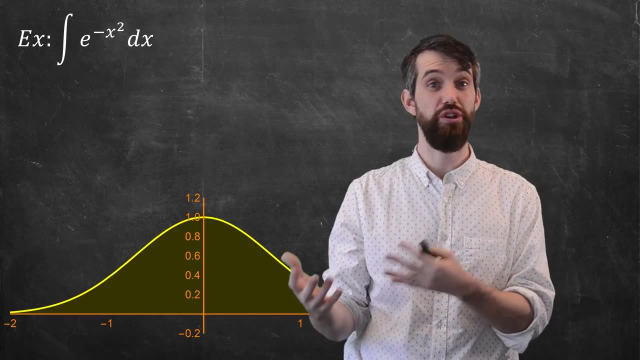 We can't, for example, do a u sub. It doesn't work out. Maybe you'd want to try an integration by parts. It's not going to be nice. In fact, it turns out that there isn't a nice answer in terms of functions like e to the x, and polynomials and trigonometry and so on. 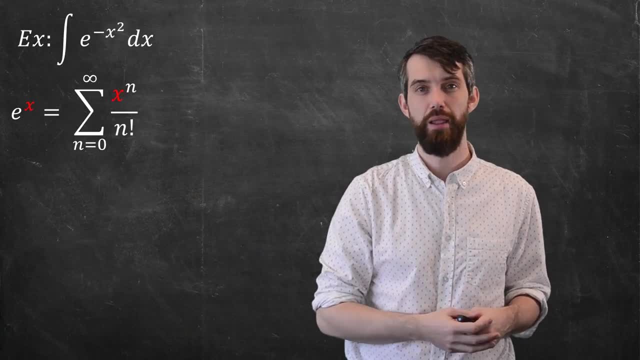 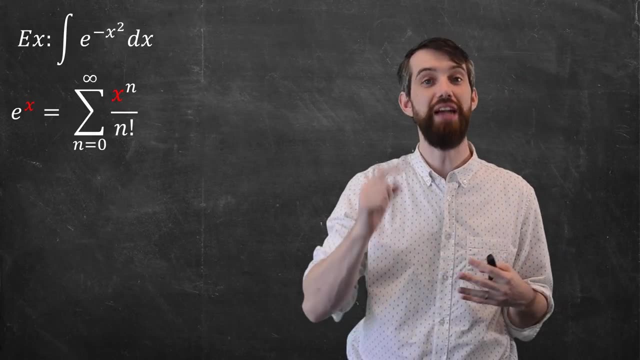 But we can use series, So, for example. so, for example, we know that the Taylor Series for e to the x is just this sum, from 0 to infinity, of x to the n over n factorial. Indeed, this is the Taylor Series centered about x equal to 0.. 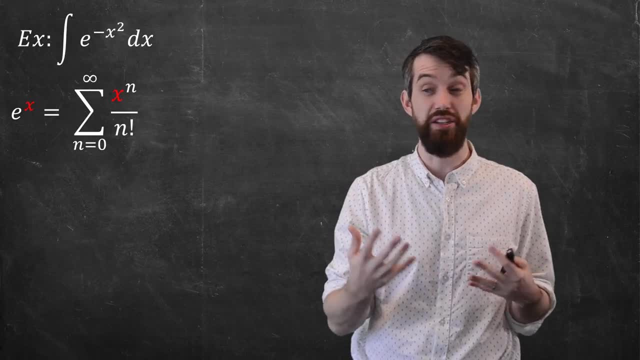 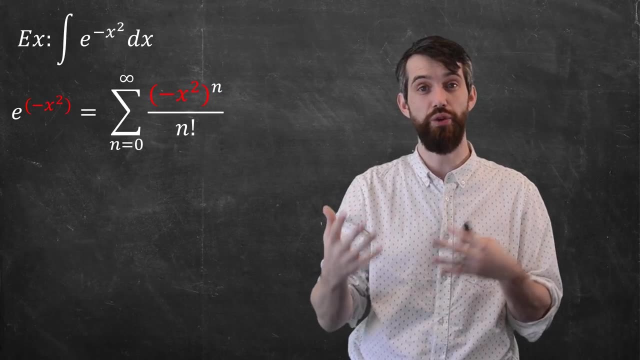 Now this is e to the x, but in my integrand I have e to the minus x squared, So let me just substitute that in, And everywhere I have an x, I'm going to replace it with a minus x squared. Now I'm doing the integral of this thing. 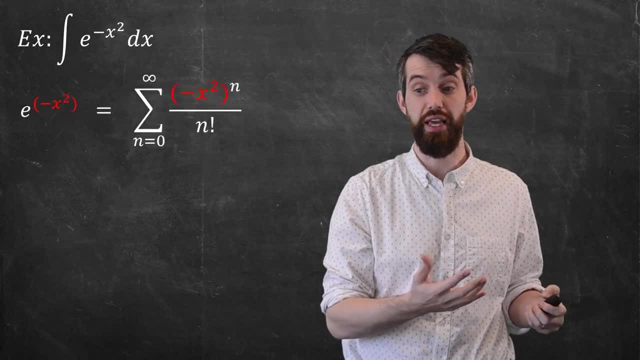 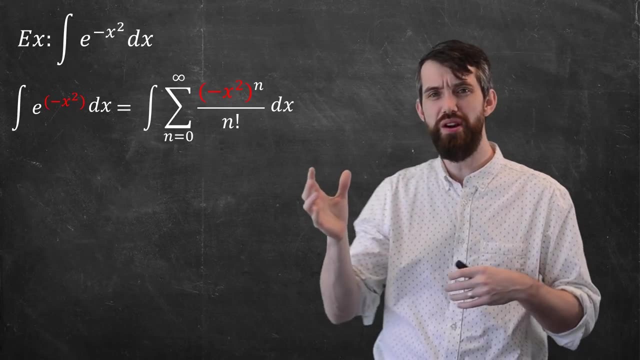 So let me go and take the integral of both sides of these things, dx, And then I'm going to do one final, just little bit of cleanup job. You see how I've got the minus x squared all to the power of n. Let me take the minus sign out of that. 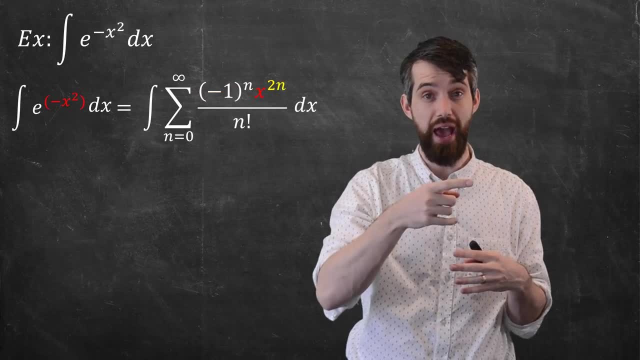 And so if I transform this, what I'm going to have is a minus 1 to the n and then an x to the 2n. Now, what I'm going to do with this Taylor Series is I'm going to integrate it. 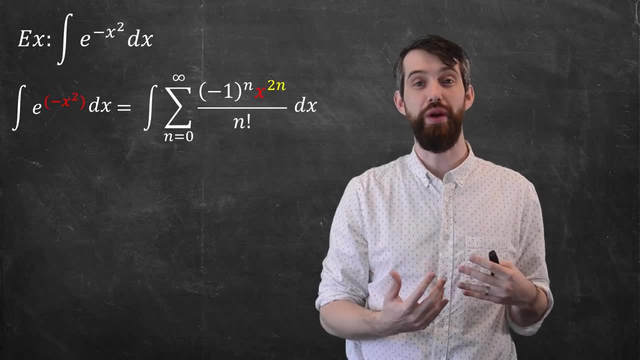 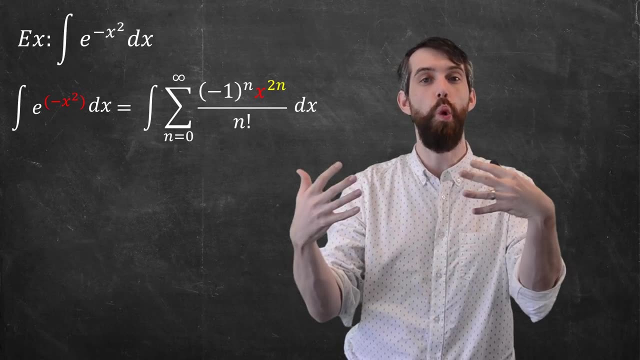 term by term, and that is in effect. I'm integrating some constant times: x to the 2n. What happens to that? x to the 2n will go to x to the 2n plus 1 divided by 2n plus 1,. 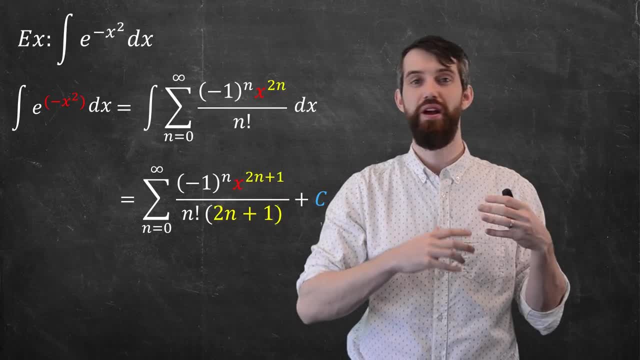 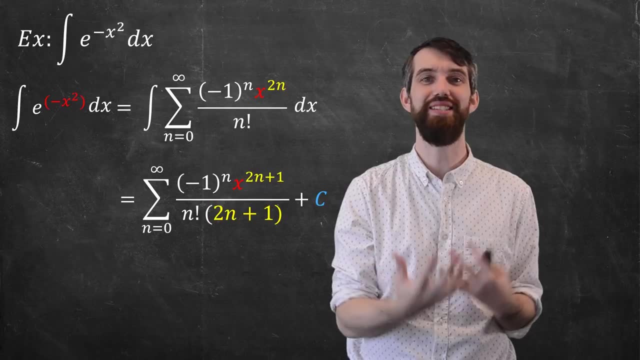 which is going to give me this particular series, the sum of minus 1 to the n over n factorial, and then an x to the 2n plus 1, and then you divide out by the 2n plus 1.. And finally, because it's an indefinite integral, you have to add a plus c. 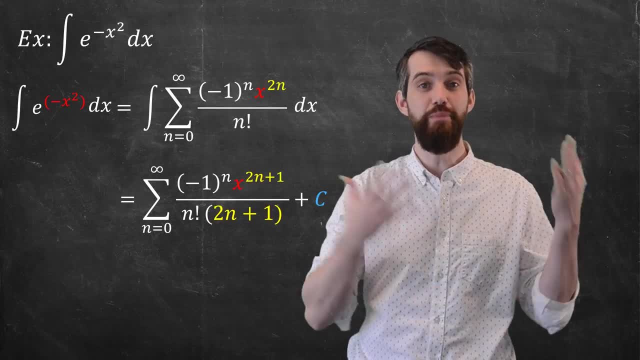 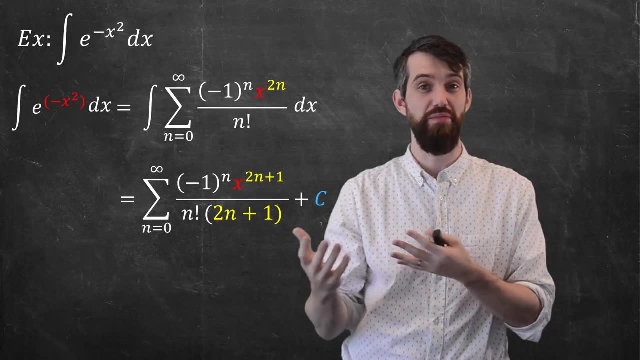 So that's a perfectly acceptable answer. We now have a power series. We now have a power series answer to this integral of e to the minus x squared. If we wanted to, we could give this collection a name whatever you prefer. You could call it after yourself, if you so wish. 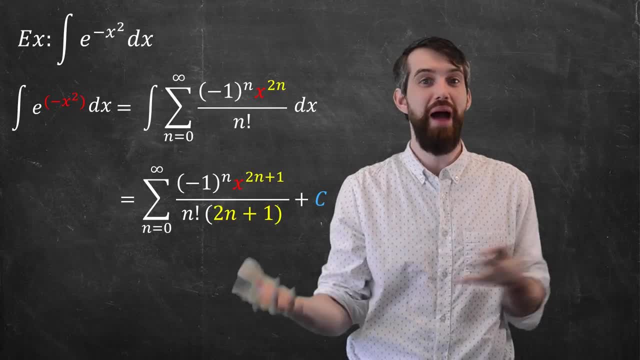 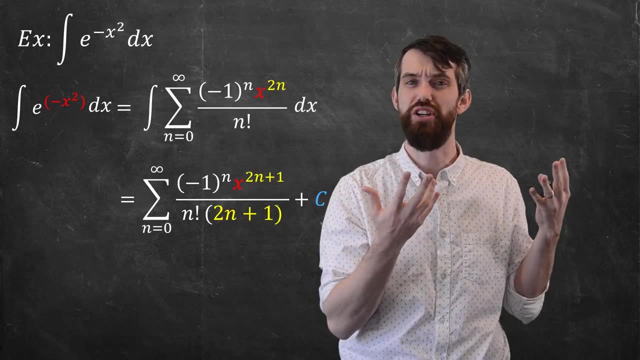 The only reason it doesn't have a name is because, as a group of mathematicians, we haven't ended up agreeing on one, the way we agreed on a name for the special function e to the x and a special function sine of x, And then, if I want to, I can also do a definite integral here. 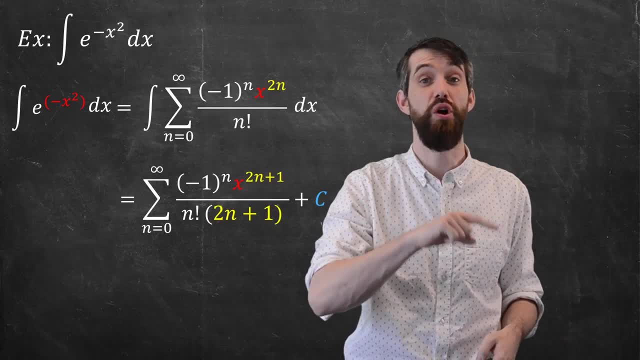 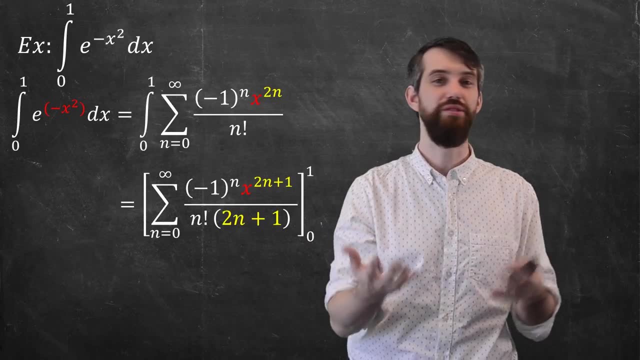 So everywhere that I've got my indefinite integral, I'm going to place it with a 0 up to 1. And indeed, when I have my final series, I evaluate it from 0 up to 1.. Plugging in 0 doesn't do anything. 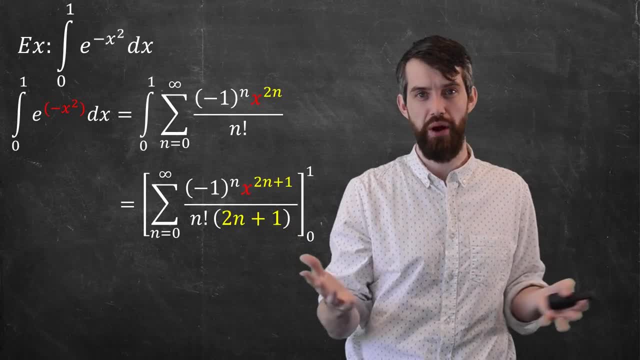 x to the 2n plus 1, when x is 0, is just 0,, so that's all 0. And if I plug in 1, the x portions are going to go away. 1 to the 2n plus 1 is 1.. 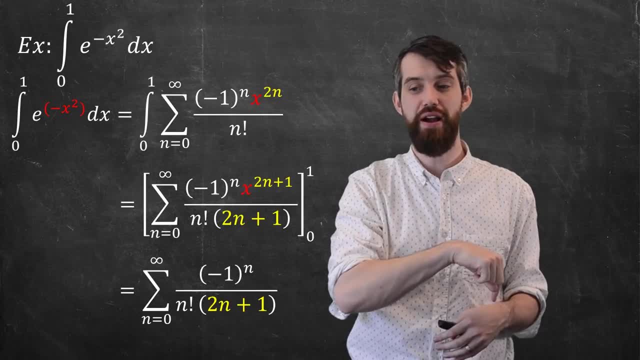 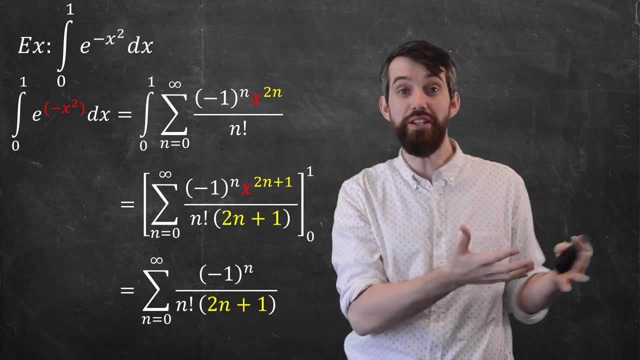 And that just leaves me behind minus 1 to the n over the n factorial and over that 2n plus 1.. And this is a perfectly acceptable answer if, in your application, you needed to approximate this integral as accurately as you so wished. 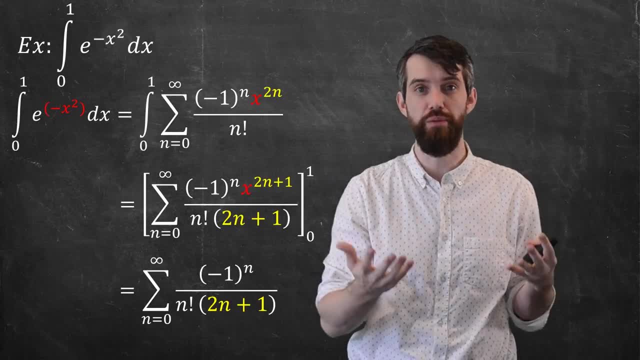 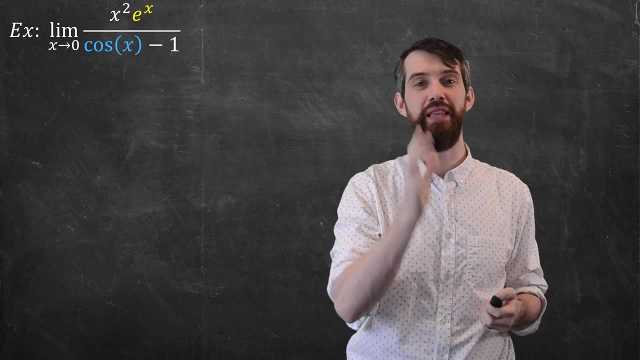 Well, You could go and take the first 10 or 100 or a million terms, however many terms that you needed for your level of accuracy. All right, so that's an integration example. Next up, let's look at a limit example. 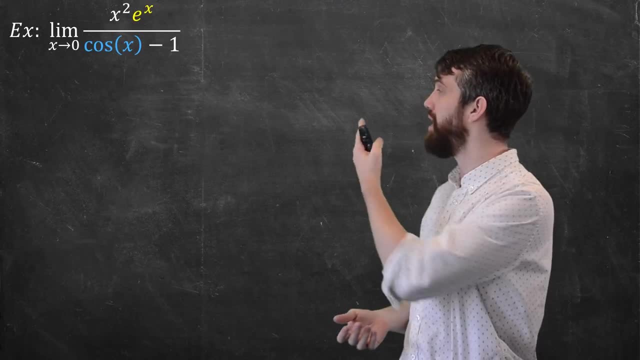 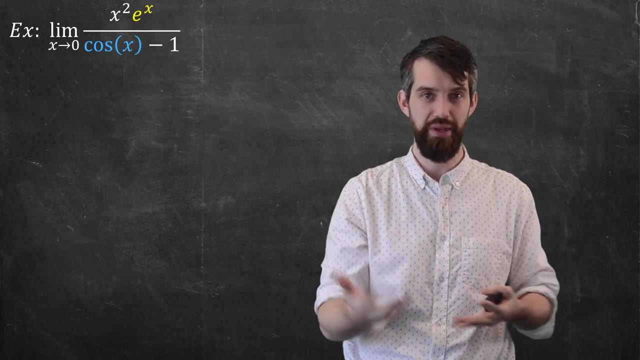 So in this example I have an indeterminate form. If I just plugged in x equal to 0, I have 0 on the top and 0 on the bottom, And what we learned back in Calculus 1 is that in those scenarios you can do L'Hopital's. 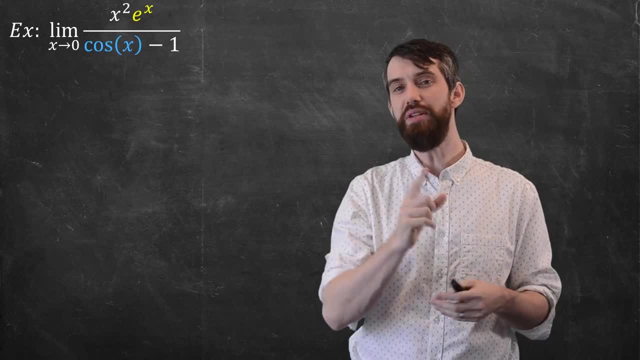 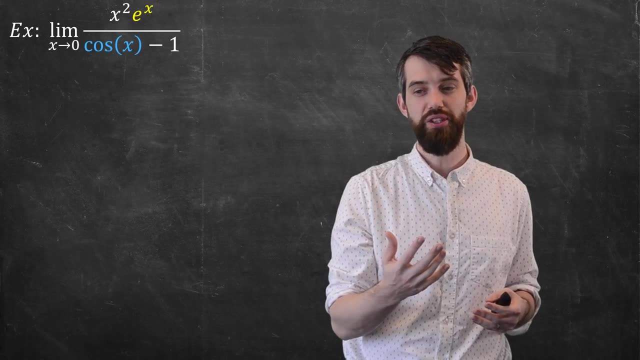 rule. In this case, maybe you have to do it once and twice, And L'Hopital's rule often works. Indeed, it works in this particular example, But I'm going to show you how I can do it with a Taylor series. 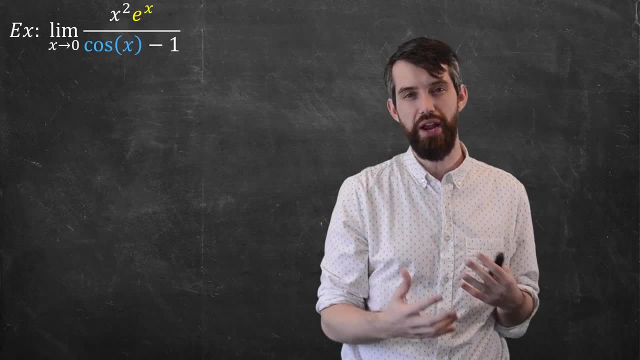 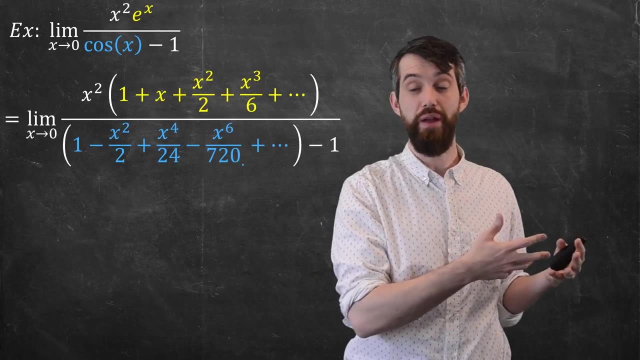 So in this expression I've got this e to the x and the cosine of x, and both of those have series expansions, which is to say if I go and plug them in, so my x squared is still at the front, but in place of e to the x I've put its series and in place of cosine. 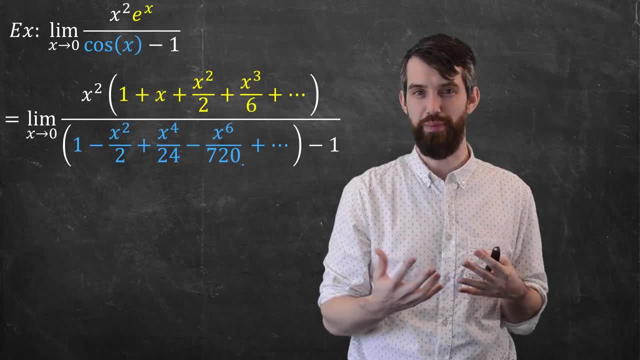 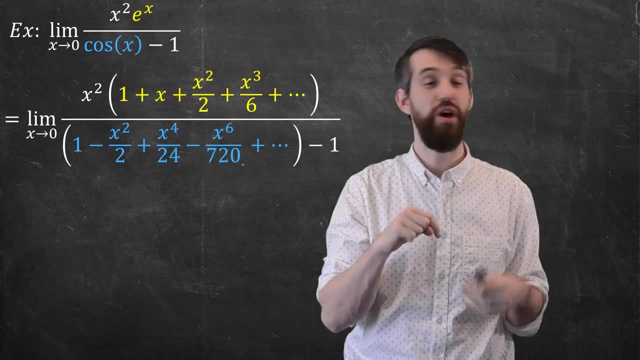 of x. I've put its series. Let me try to clean this up a little bit. So the numerator: I have an x squared multiplied by a whole series. So let me just put those together and in the denominator I've got a plus 1 and a minus. 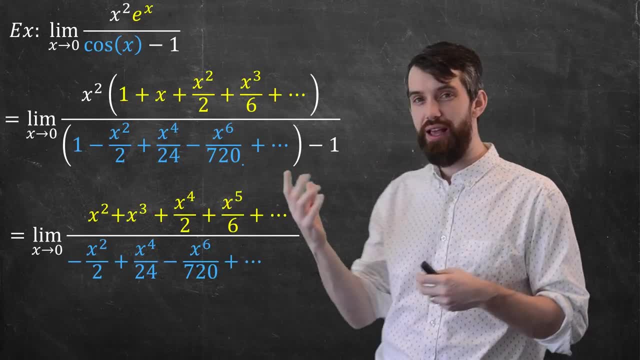 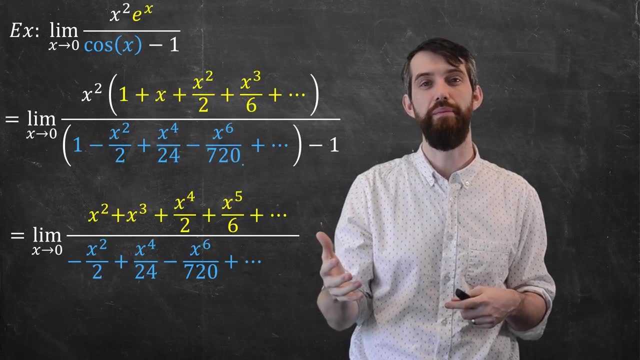 1. That is- I'm going to have this expression- an x squared and higher order terms on the top and a minus x squared over 2 and higher order terms on the bottom. The fact that there's higher order terms here is important because I'm setting the limit. 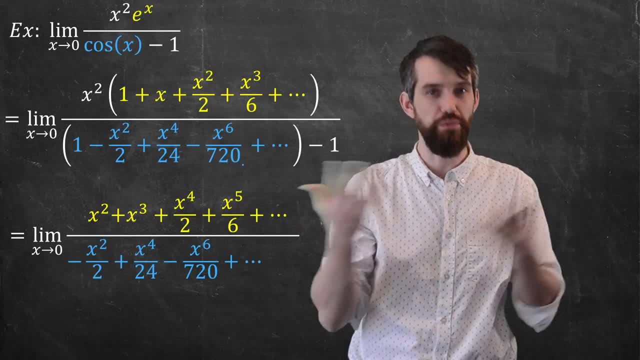 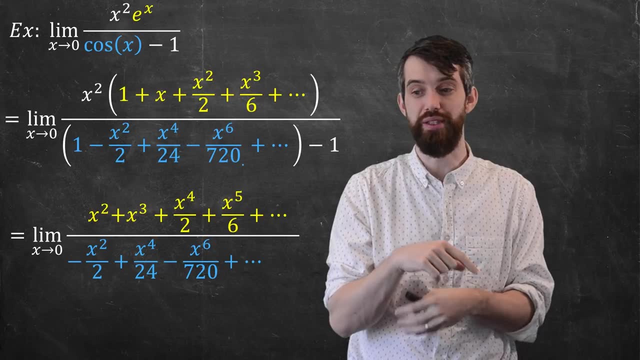 as x goes to 0, so that means that every one of these terms is going to go to 0. But the higher order terms go to 0 faster. The x cubed goes to 0 faster than x squared does. The x to the fourth goes to 0 faster than x squared does. 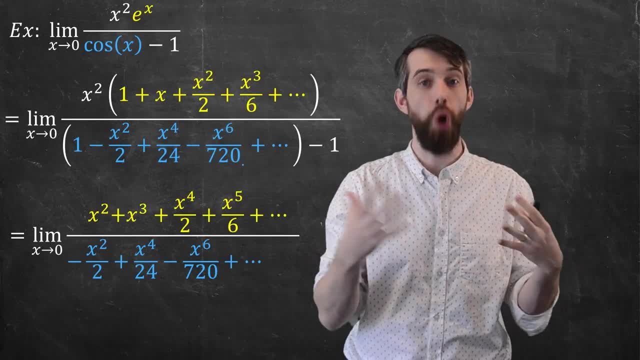 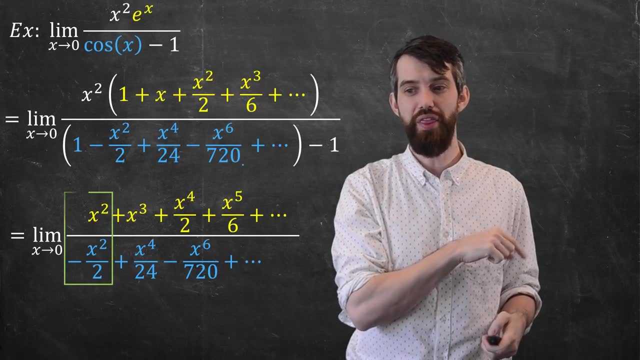 So when I look at the top and the bottom, I'm going to have this expression and I'm going to try to figure out which is going to dominate as x is going to go to 0. Well, it's those lowest order ones that do it when x is being sent to 0.. 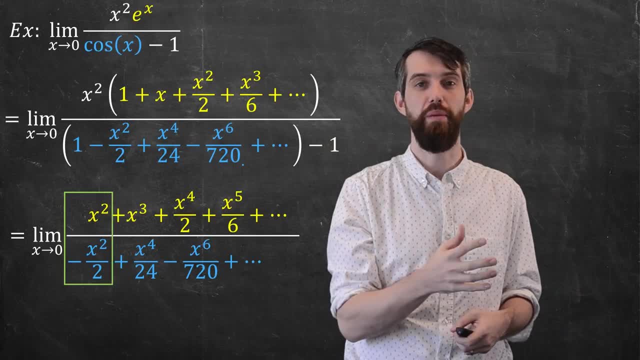 That is, the things I really want to focus on is the first term on the top and the first term on the bottom. So everything else is going to go to 0, and it's going to go 0 in a way that is faster. 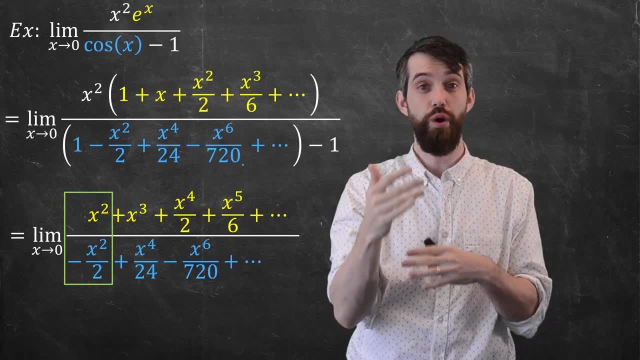 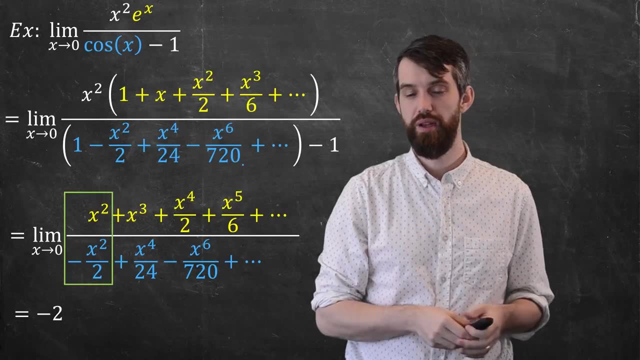 than these, But these two are going to cancel. x squared over. x squared cancels and it just leaves the coefficient 1 over minus 1 half. in other words, this is equal to the value of minus 2.. So with this kind of analysis you're able to solve a whole class of limits that were 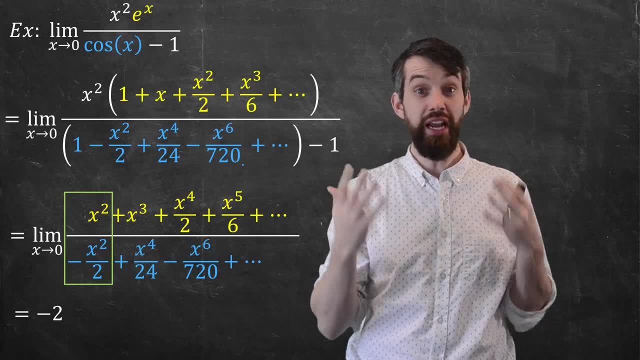 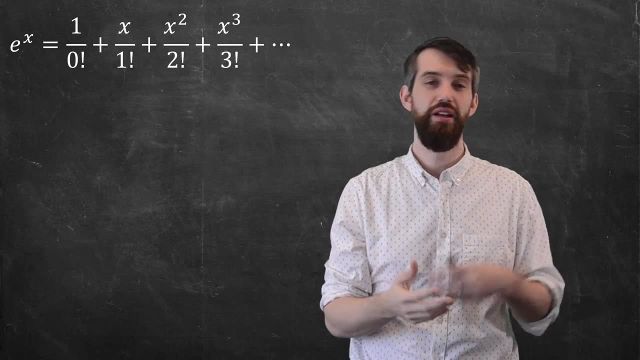 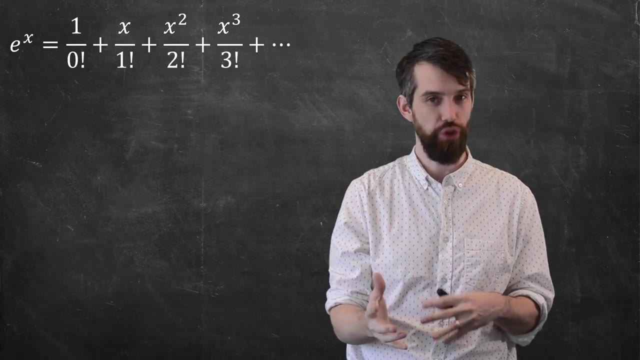 challenging before as well. Final application for Taylor series is actually going to be series themselves. So, for example, this is the Taylor series for e to the x: the 1 over 0 factorial plus x over 1 factorial, x squared over 2 factorial plus x cubed over 3 factorial, and so on. 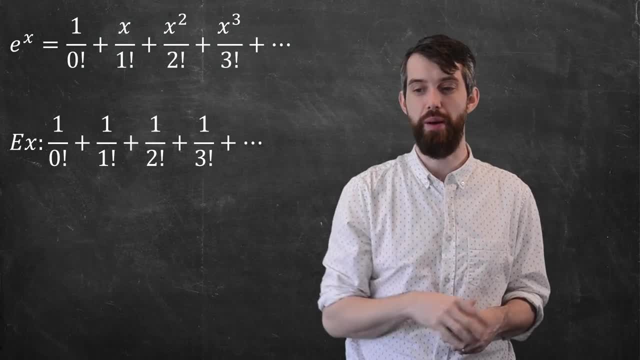 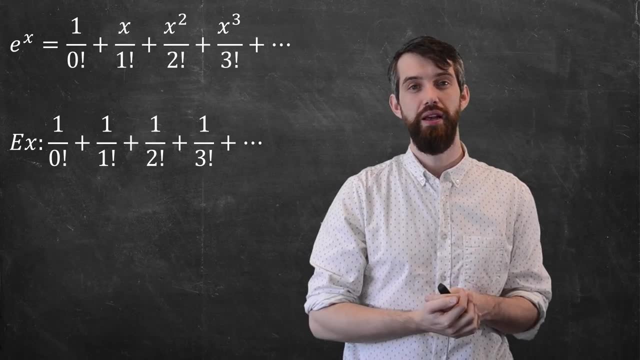 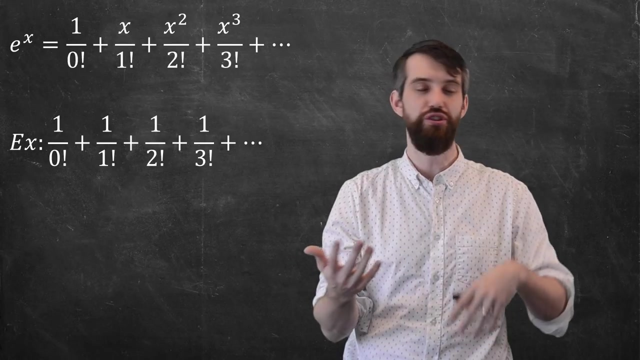 Well, what if, instead, I was giving you this problem, this expression where there is no x, It's just some particular series. Now, if this was earlier on in calculus 2, we would have said, well, does it converge or does it diverge? and you could have used a ratio test or maybe a comparison test. 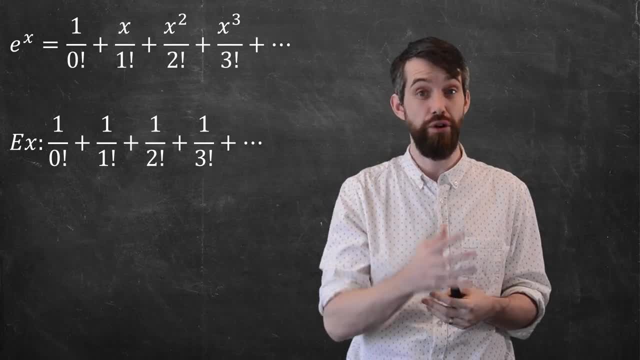 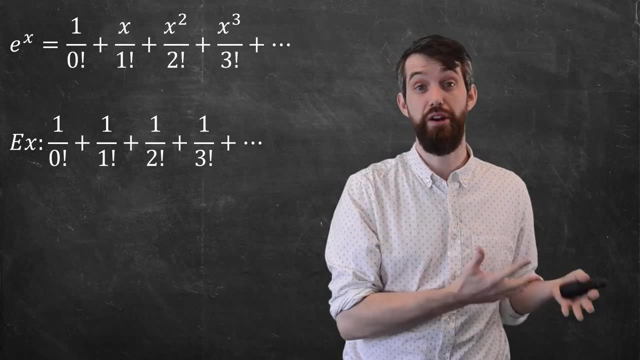 There were a bunch of options, but you would have deduced that, yes, it converges by some particular test, But what does it converge to? That was an open problem, or at least would have been an open problem before. But now, if I look at this example, this example is nothing but e to the x where I've plugged. 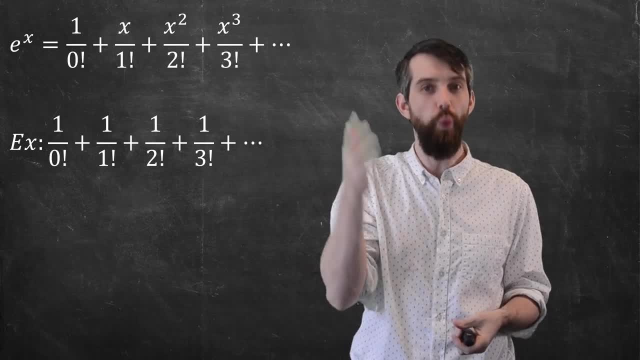 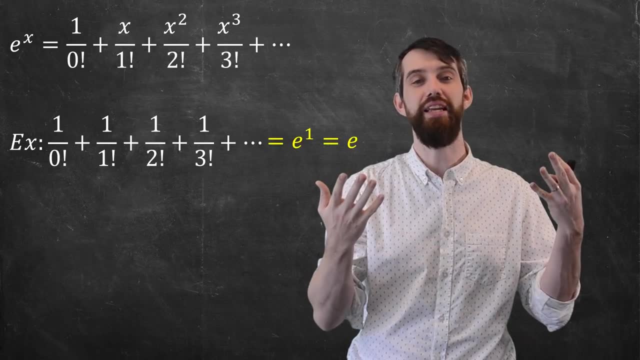 in x equal to 1 everywhere. Those entire numerators are now all 1.. That's me plugging in x equal to 1.. So what is this series? Well, it's just whatever e to the 1 is, that is, it is e. 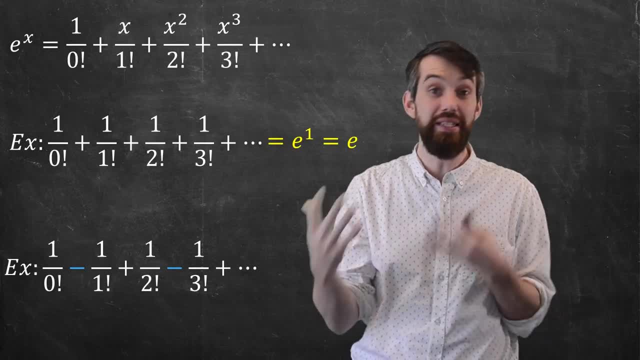 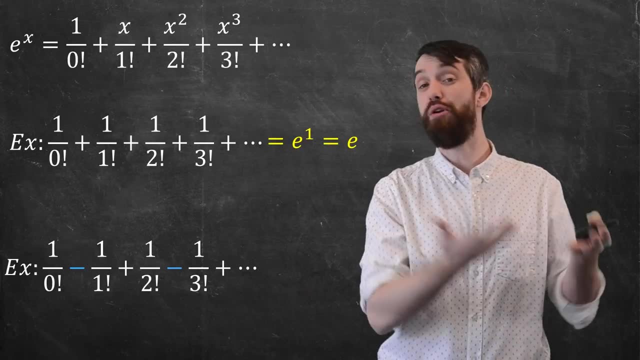 Or if I slightly change things up, if I consider the same basic example, but I put some plus minus, plus minus things again. if we were doing a convergence test, maybe you would use- oh, I don't know- the alternating series test and deduce that it converged. 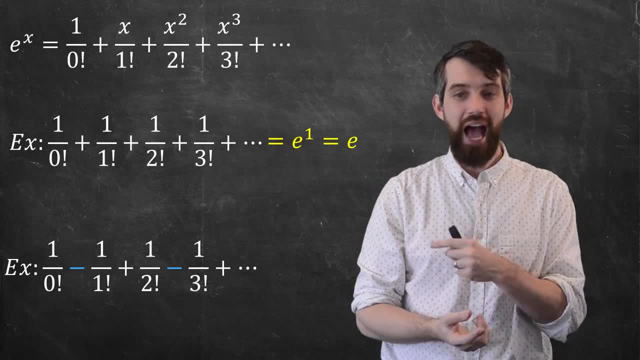 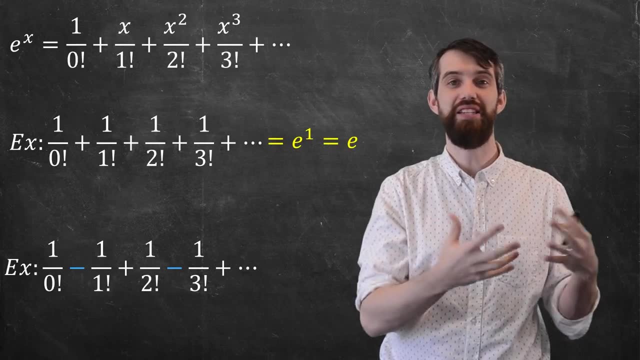 But what did it converge to? Well, this thing is exactly e to the x, but I am plugging in not x equal to 1.. But x equal to minus 1, indeed, for, like the x and x cubed, and x to the fifth and odd power. 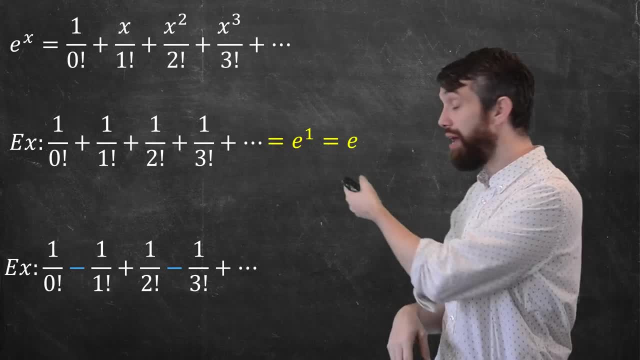 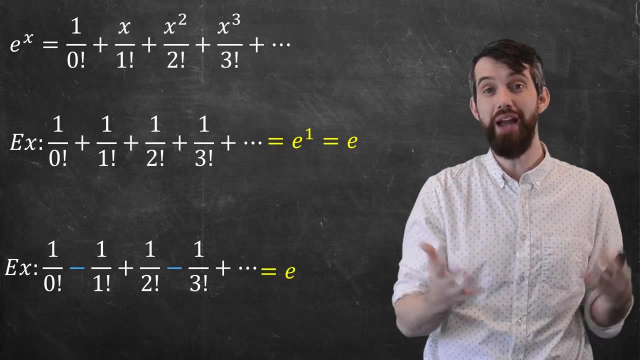 terms, Putting in minus 1 is going to stick out a negative And for all the even power terms, putting in minus 1 is not going to do anything. It's going to become positive. So this is just e to the power of minus 1, aka 1 over e. 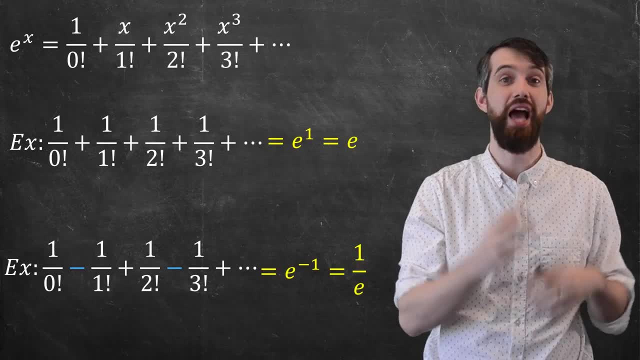 So in this video we've seen these three different ways that I can apply Taylor series to problems from the past in our development of calculus.